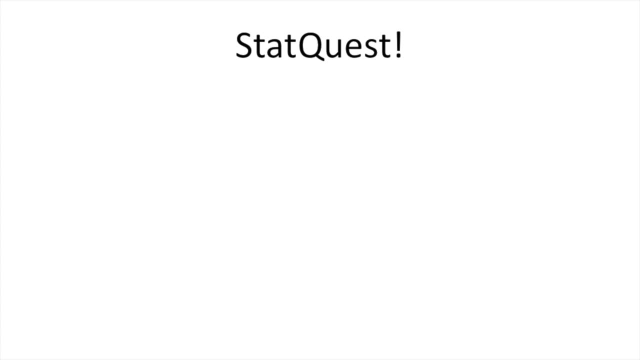 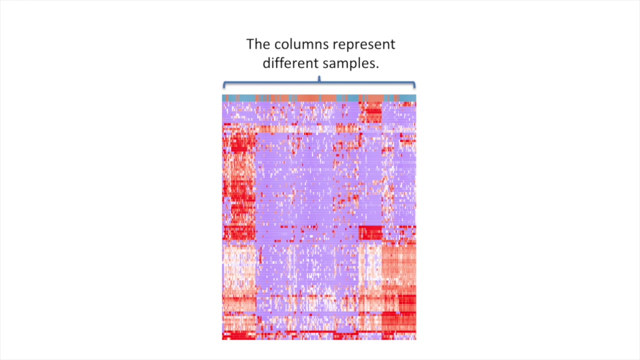 Hello and welcome to StatQuest. Today we're going to be talking about Hierarchical Clustering. Hierarchical clustering is often associated with heat maps. If you're not already familiar with what heat maps are, just know that the columns typically represent different samples and that the rows typically represent measurements. 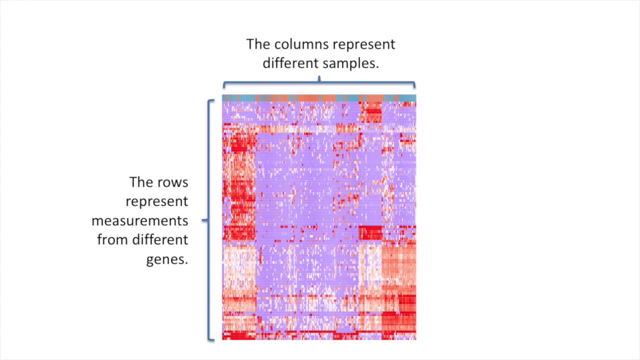 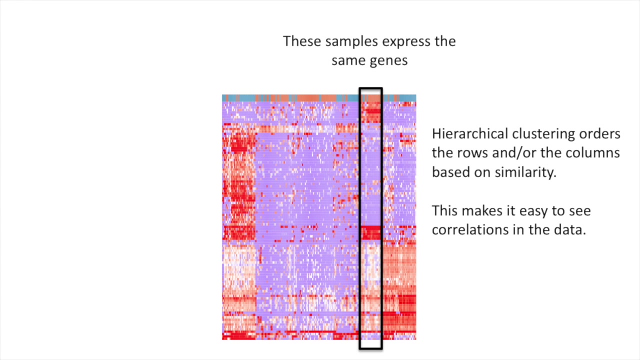 from different genes. Red typically signifies high expression of a gene, and blue or purple means lower expression for a gene. Hierarchical clustering orders the rows and or the columns based on similarity. This makes it easy to see correlations in the data. For example, these samples express: 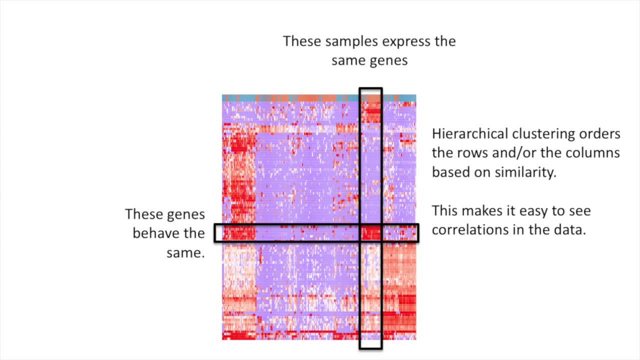 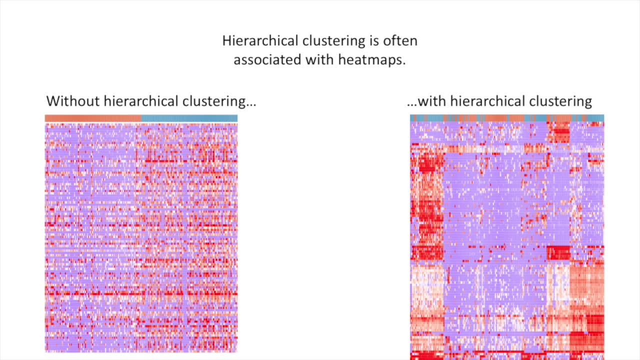 the same genes and these genes behave the same. On the left we have a heat map without hierarchical clustering and on the right we have a heat map with hierarchical clustering. So you can see that the clustering makes a big difference on how the data is presented. Heat maps often come with 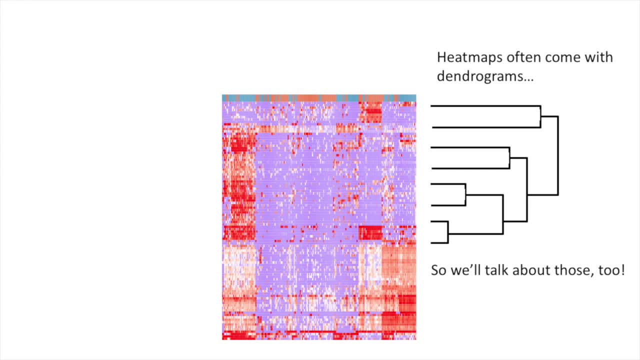 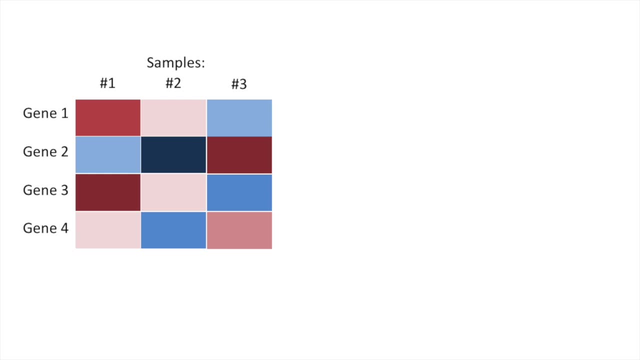 a simple heat map that has three samples and four genes, So we'll talk about those too. Let's get started. We'll start with a simple example. Here we've got a simple heat map that has three samples and four genes. For this example, we are just going to cluster or reorder the rows or the genes. 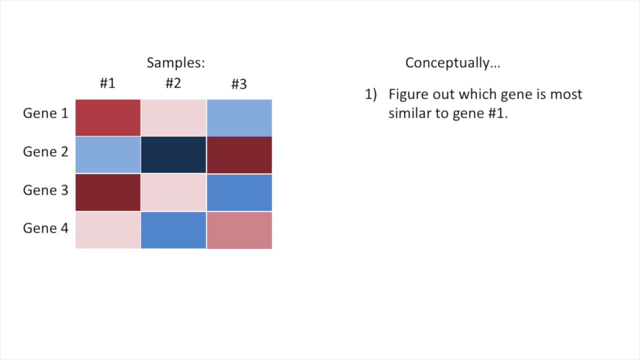 Conceptually, the first step is to figure out which gene is most similar to gene number one. Genes number one and two are different. We can tell because the colors are very different. Gene one is highly expressed in sample number one, so it has a red color. 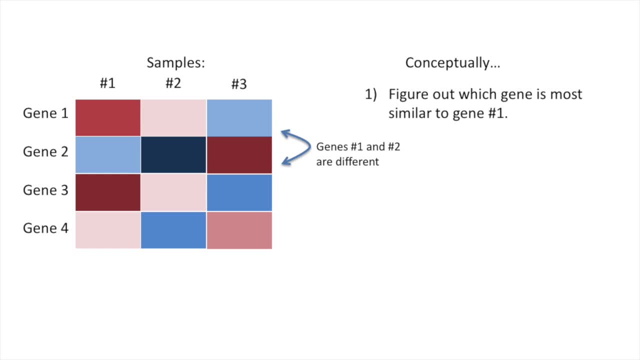 Gene two, however, is not highly expressed in sample number one, so it has a blue color. In sample number three, gene one is lowly expressed, so it's blue, and gene two is highly expressed, so it's red. In sample three, gene one and three are similar, so that means in sample one both gene one. 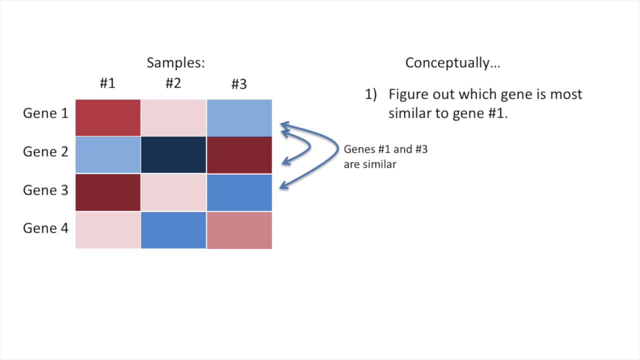 and three are red- they're highly expressed- And in sample three they're both blue, meaning they're lowly expressed. Genes one and four are also similar. However, gene number one is most similar to gene number three. So the second step is to figure out what gene is most similar to gene two. 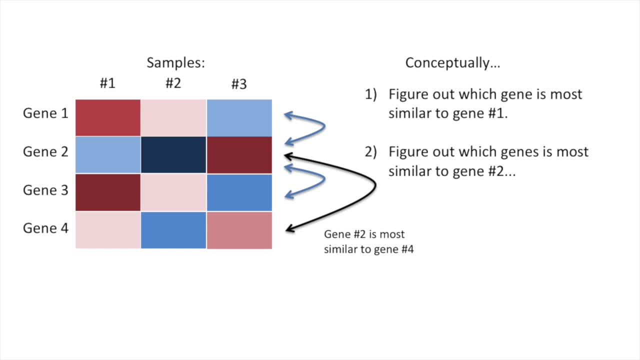 similar to gene number 2.. So we do all the comparisons and we see that gene number 2 is most similar to gene number 4.. And then we do the same thing for gene number 3 and then gene number 4.. In step number 3, we look at the different. 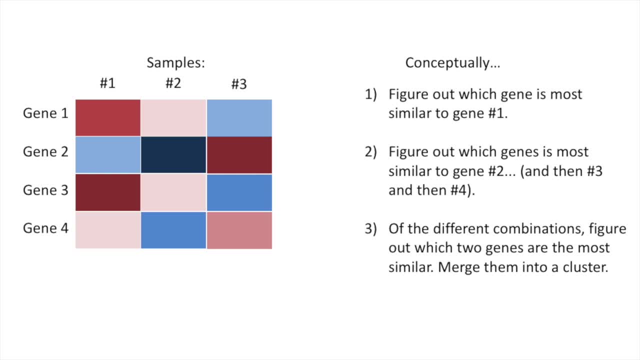 combinations and figure out which two genes are the most similar. Once we've done that, we merge them into a cluster. In this case, genes number 1 and 3 are more similar than any other combination of genes, so genes 1 and 3 are now. 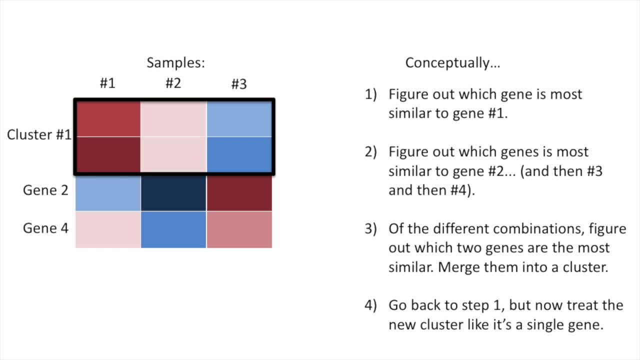 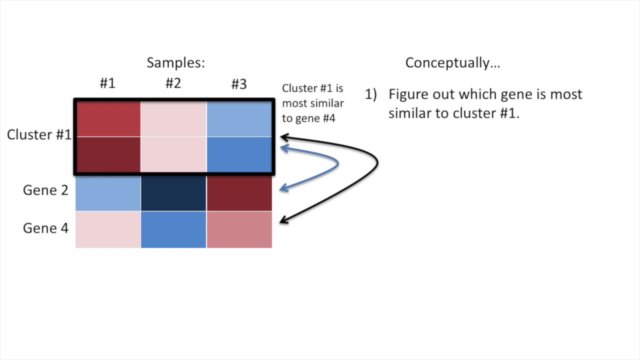 cluster number one. Step 4, go back to step 1, but now treat the new cluster like it's a single gene. So in step 1, we figure out which gene is most similar to cluster number one. Cluster number one is most similar to gene number four, And we figure out which. 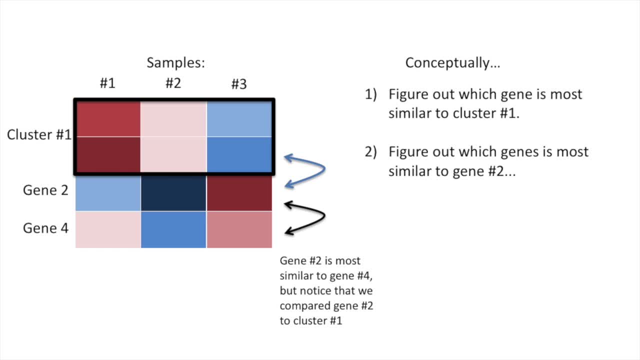 which gene is most similar to gene number 2.. In this case, gene number 2 is most similar to gene number 4, but notice that we compared gene number 2 to cluster number 1.. And then we do the same thing for gene number 4.. Of the different combinations, figure out which. 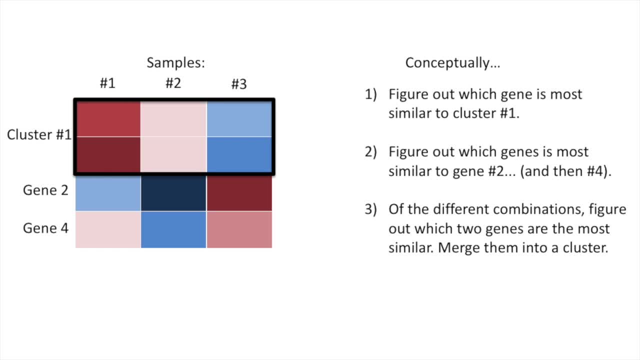 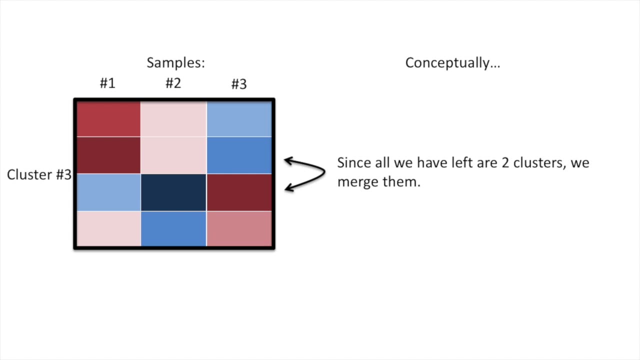 two genes are the most similar. Now merge them into a cluster. In this case, genes 2 and 4 are the most similar combination, So we've merged them into a cluster. Now we go back to step 1.. However, since all we have left are two clusters, we merge them Bam. 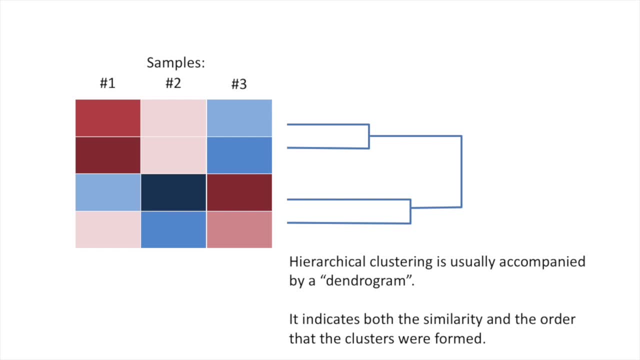 We're all done. Hierarchical clustering is usually accompanied by a dendrogram. It indicates both the similarity and the order that the clusters were formed. Cluster number 1 was formed first and is most similar. It has the shortest branch. Cluster number 2 was second and is the second most similar. It has the second shortest branch. 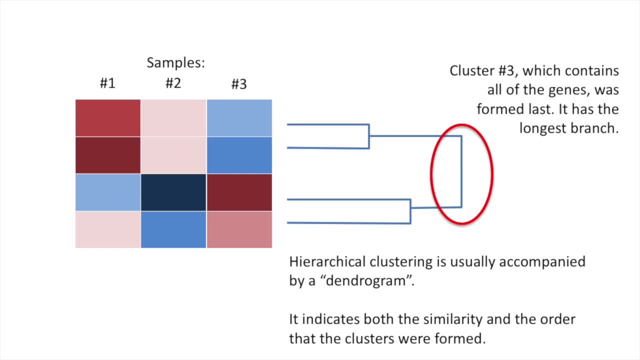 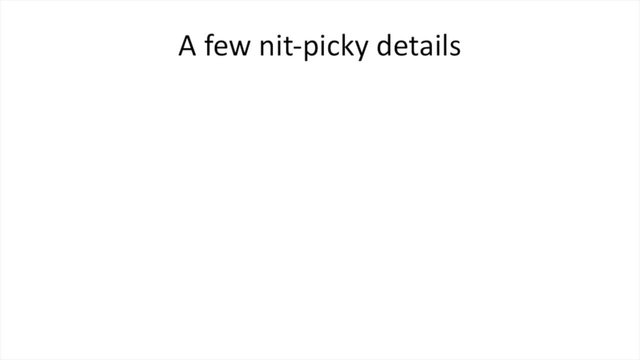 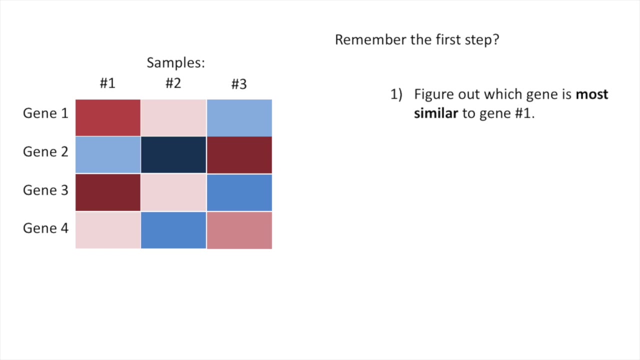 Cluster number 3,, which contains all of the genes, was formed last. It has the second longest branch. The first cluster is the longest branch. Now let's go over a few nit-picky details. Remember the first step: figure out which gene is most similar to gene number 1? Well, 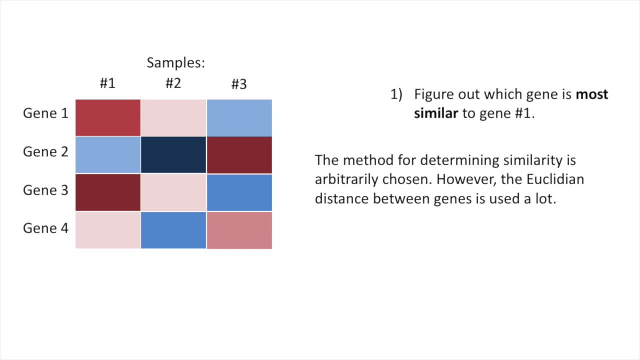 we have to define what most similar means. The method for determining similarity is arbitrarily chosen. However, the Euclidean distance between jeans is used a lot. Let's look at an example example. We'll use a very simple heat map that just has two samples and two genes. 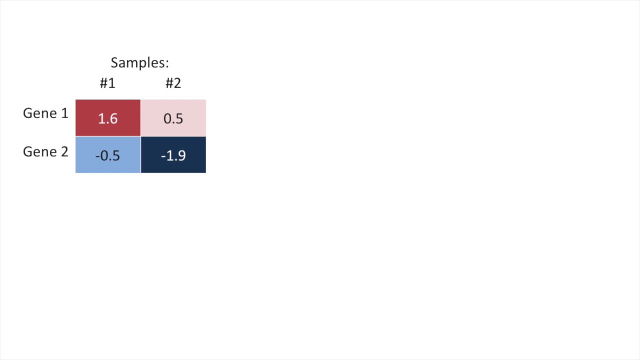 Now we're displaying the values that underlie the colors that we have in the heat map. The Euclidean distance between genes 1 and 2 is just the square root of the difference in sample number 1 squared, plus the difference in sample number 2 squared. Here we'll just plug in the values for sample number 1.. We have 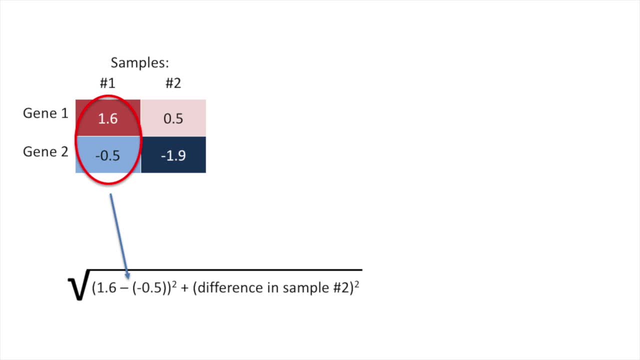 1.6 minus negative 0.5.. Now let's plug in the values to calculate the difference in sample number 2.. We have 0.5 minus negative 1.9.. Doing the subtraction gives us the square root of 2.1 squared plus 2.4 squared. 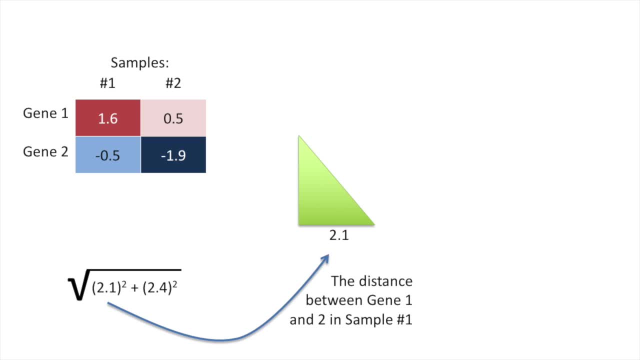 We. We can think of these values, within the parentheses, as sides on a triangle. So on the x-axis we have the distance between gene 1 and gene 2 in sample number 1.. And on the y-axis we have the distance between gene 1 and 2 in sample number 2.. 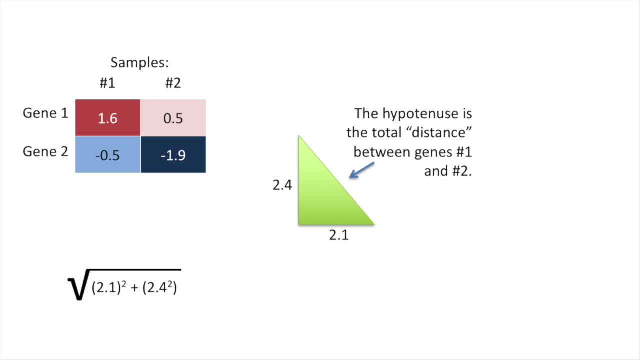 The hypotenuse is the distance between genes 1 and 2.. The Pythagorean Theorem says that the hypotenuse equals the square root of x-squared plus y-squared. In this case, that means the square root of 2.1-squared plus 2.4-squared. 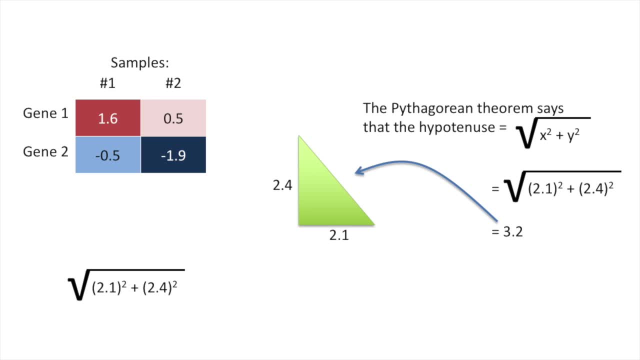 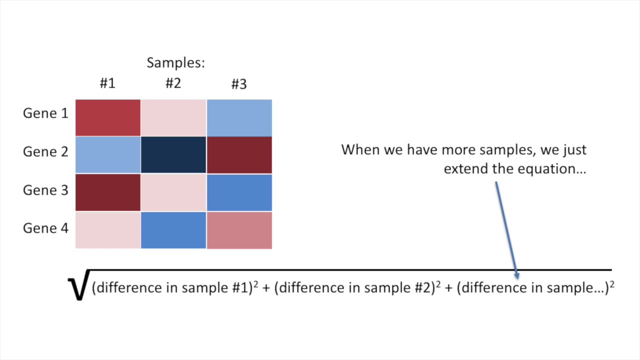 And that gives us 3.2, the distance between gene number 1 and gene number 2. When we have more samples, we just extend the equation. It's no big deal. The Euclidean distance is just 1.2.. 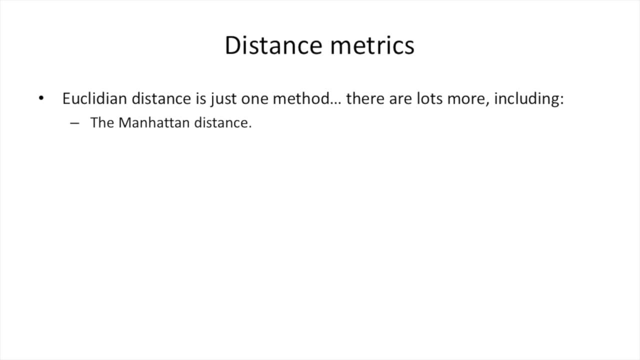 One method. There are lots more, including the Manhattan distance. The Manhattan distance is just the absolute value of the differences. So instead of squaring the differences and then taking the square root, all we do is take the absolute value of the differences. 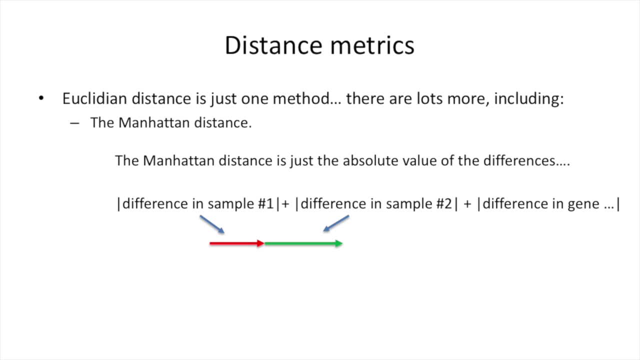 We can think of the Manhattan distance in geometric terms by imagining that each difference is a line segment. If we take all those line segments And put them together- Head to tail, head to tail- And then add that total length of all those line segments together, 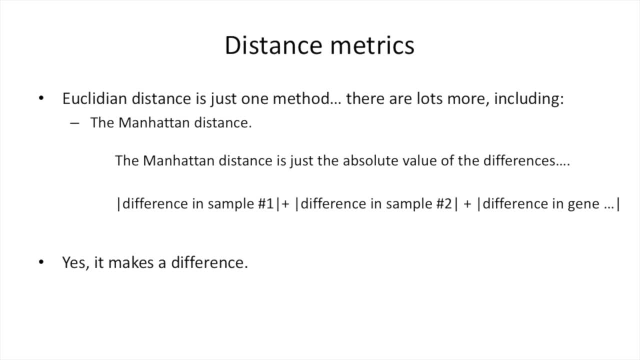 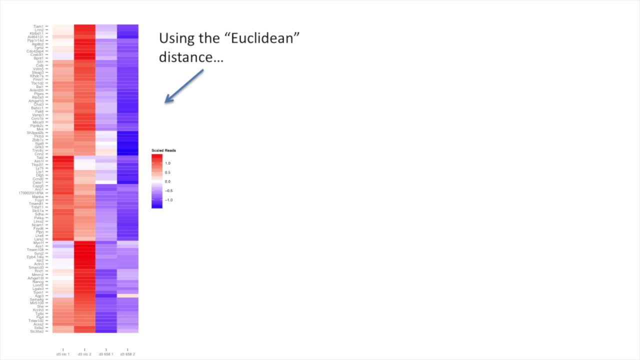 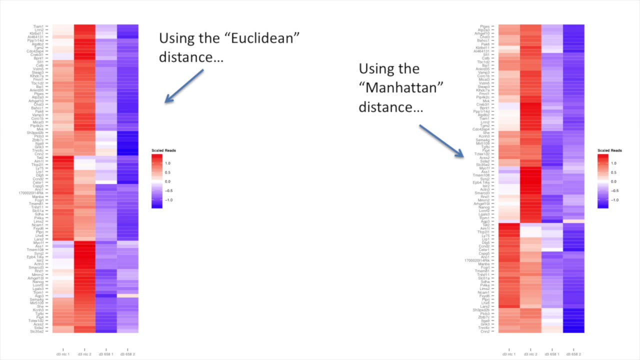 That's the Manhattan distance. Yes, It makes a difference, Wah wah. Here's a heat map drawn using the Euclidean distance And here's the same information drawn as a heat map, but now we're using the Manhattan distance. The heat maps are very similar, but there are also a few differences. 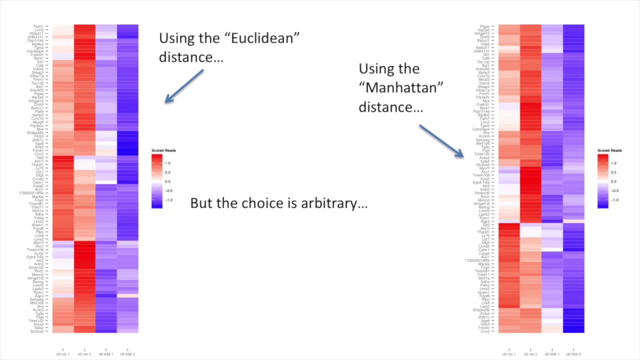 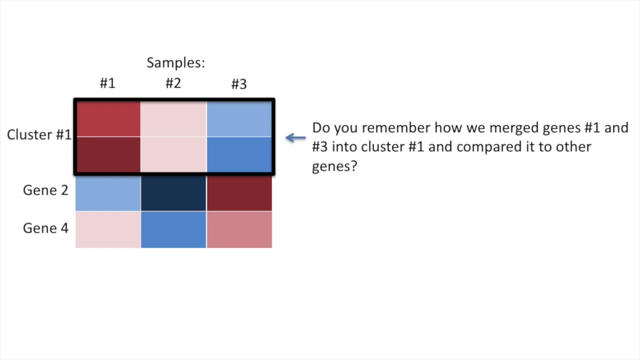 The choice and distance metric is arbitrary. Wah wah. There is no biological or physical reason to choose one and not the other. Pick the one that gives you more insight into your data. Now, do you remember how we merged genes 1 and 3 into cluster number 1 and compared it? 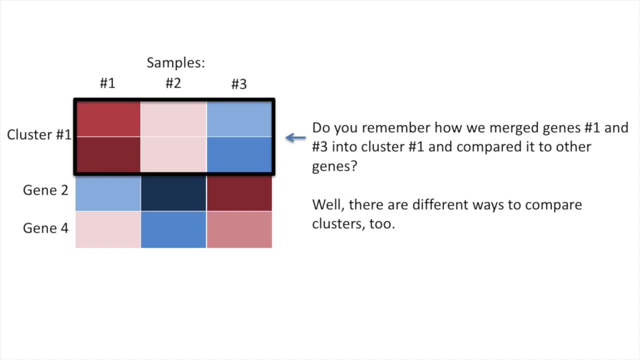 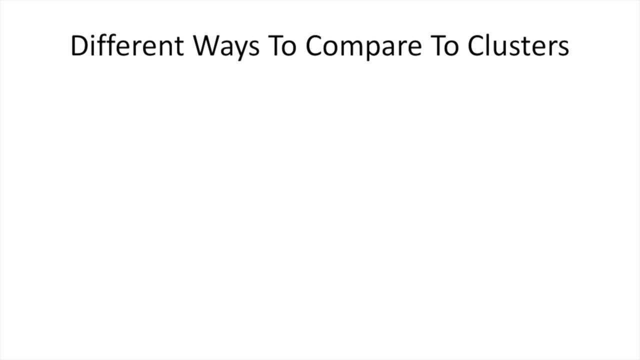 to other genes. Well, there are different ways to compare clusters too. One simple idea is to use the average of the measurements from each sample, But there are lots more, And these have effect on clustering as well. So let's talk about the different ways to compare clusters.